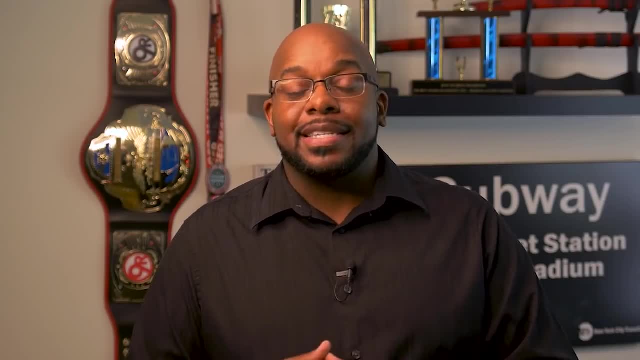 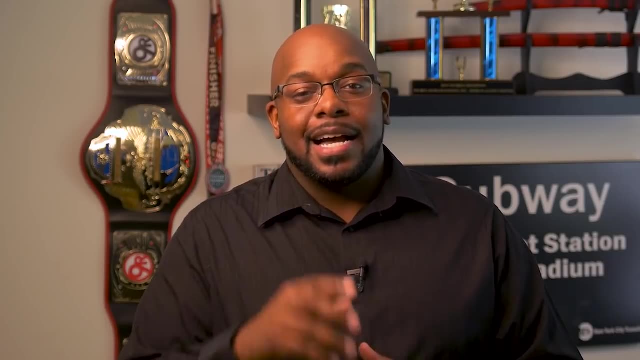 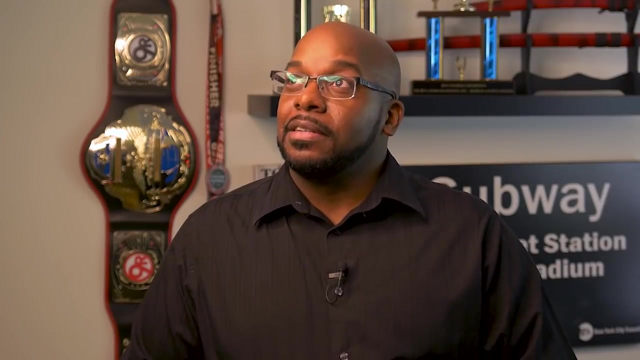 which introduces students to many of the essential skills and disciplines in the tech industry, including design, development, engineering and more. For a limited time, you can enroll in the learning track for just $5. That's 80% off- 80%. Check out the link in the description. 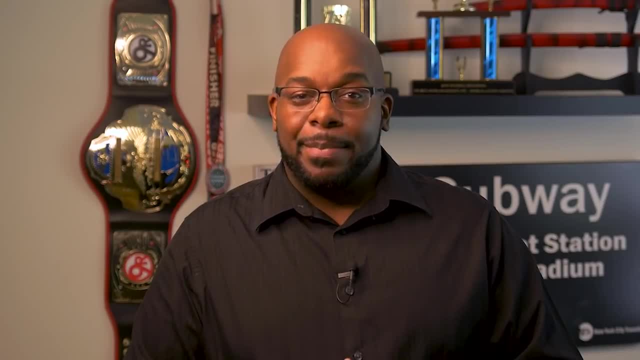 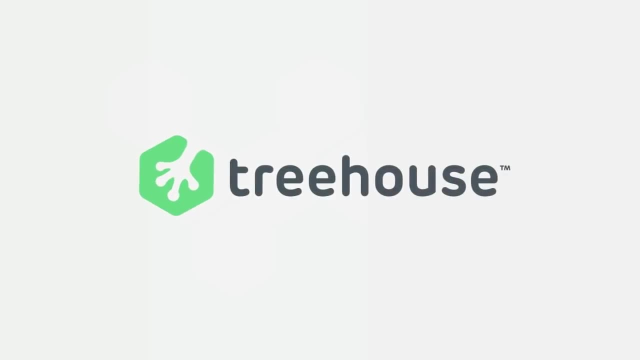 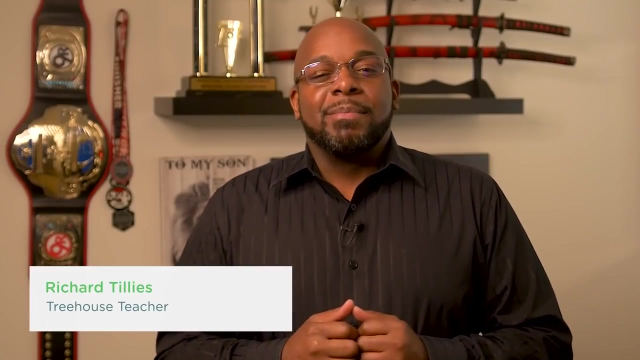 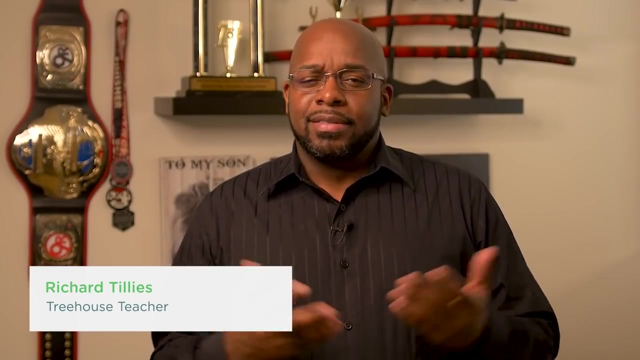 to learn more and get your discount. Happy learning. Hello world, My name is Richard, I'm an instructor at Treehouse and my background is computer science. Your first question might be: what exactly is computer science? Is it the science of working? 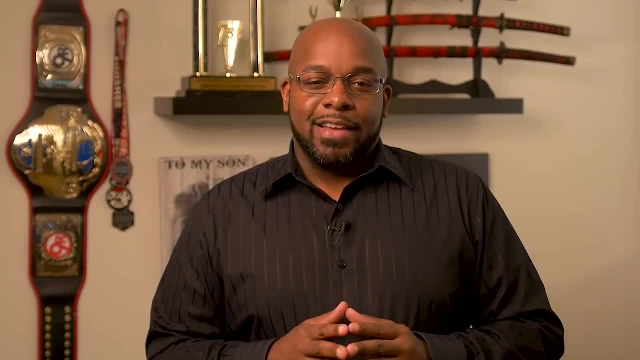 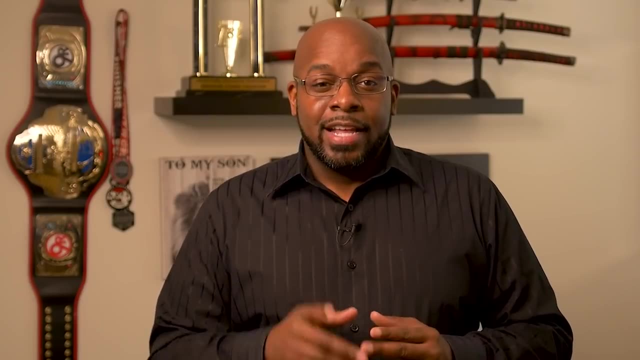 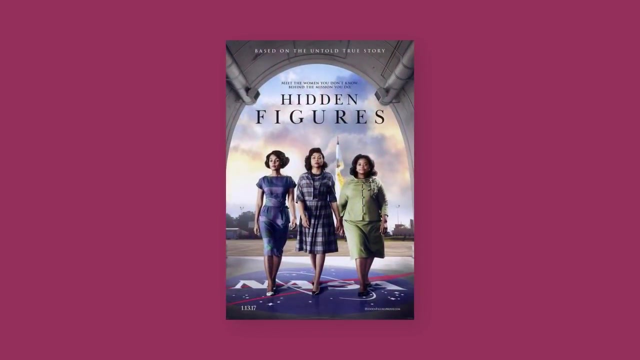 with computers? Well, there's no set definition. It seems that every major university and computing organization has their own take on it. To help us define computer science, consider the Oscar-nominated film Hidden Figures, released in 2016.. It was the true story of Black. 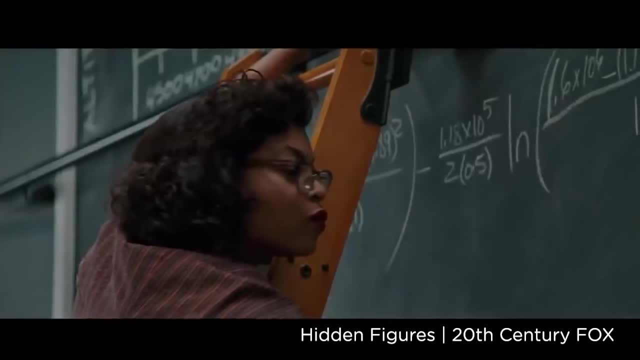 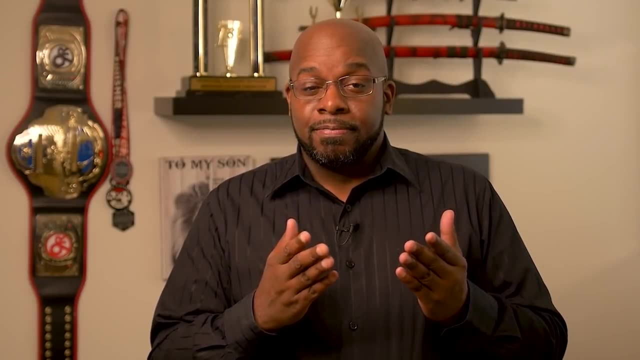 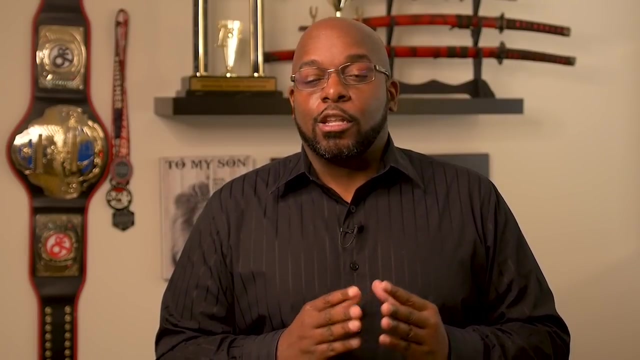 women who were hired at NASA and who were hired to do the work of computer science. They were hired to perform complex mathematical calculations for upcoming space missions. Their job title: Computers. So the term computer science doesn't necessarily refer to this machine we call a computer, because the term existed long before computers were widely available. 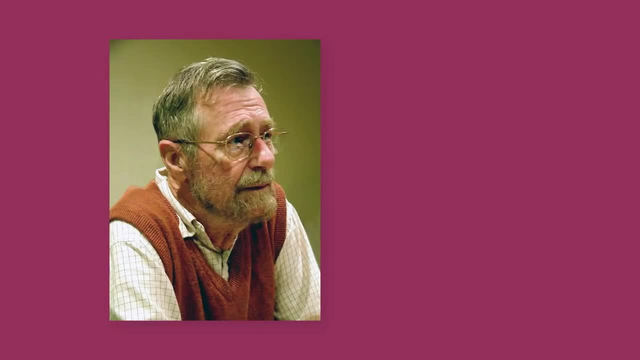 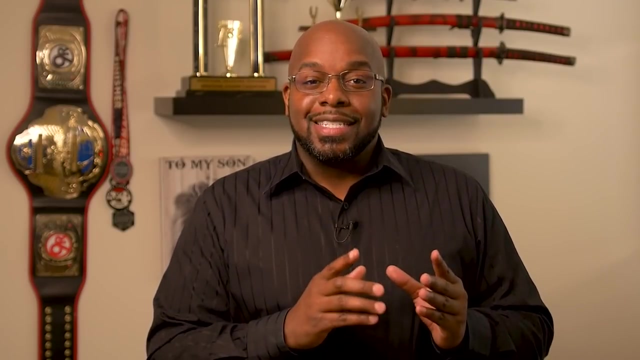 In fact, Edska Dykstra, an influential figure in the early days of the discipline, once stated that computer science is no more about computers than astronomy is about telescopes. It has been argued that a more appropriate term might be computing science, although 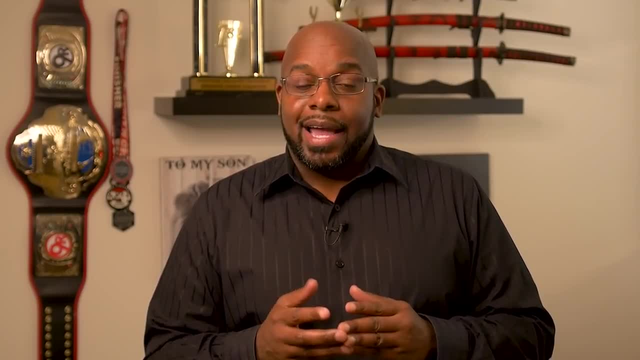 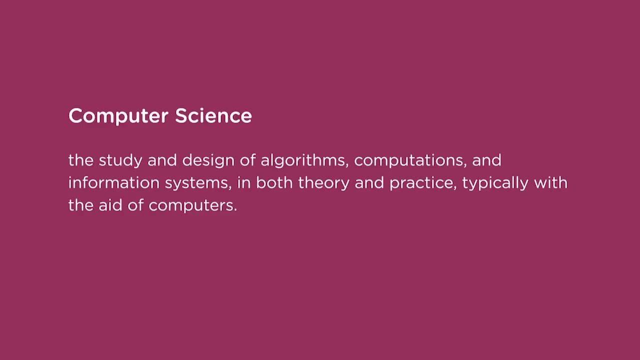 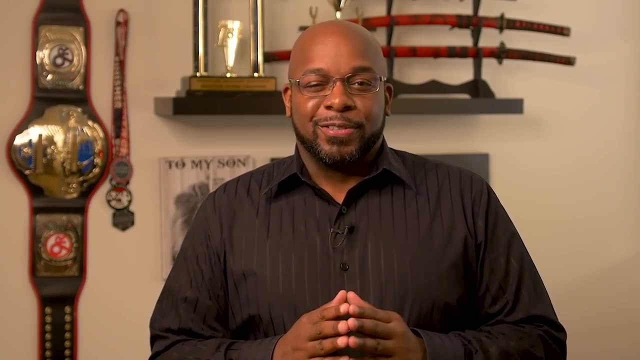 most of the work in the modern age is done for and by computers. So here's our definition: Computer science is the study and design of algorithms, computations and information systems, in both theory and practice, typically with the aid of computers. I know that's a mouthful. As we move forward, we will provide more understanding of the term. 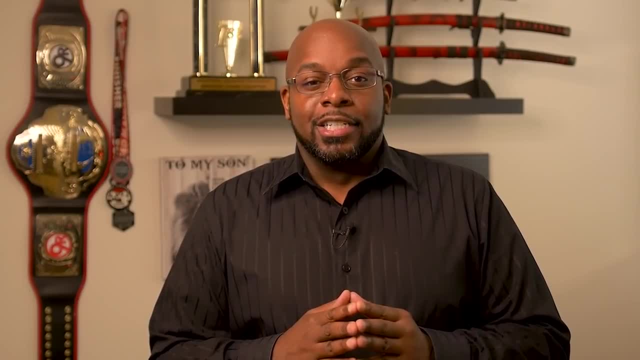 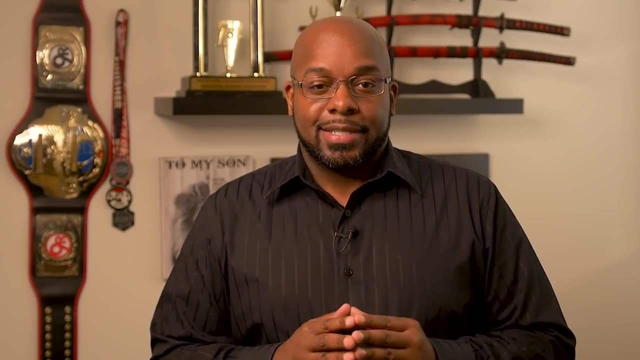 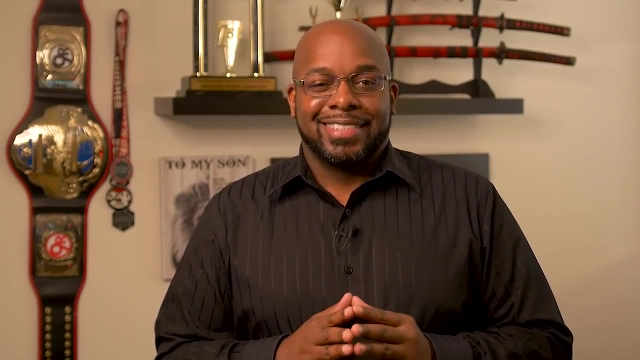 computer science as you begin this new journey. Just like telescopes are tools in the study of astronomy, computers are tools in computer science. In the next video we will unpack the history of computers and the internet. See you there. Let's talk a little history. It's hard to know where you're going if you don't. 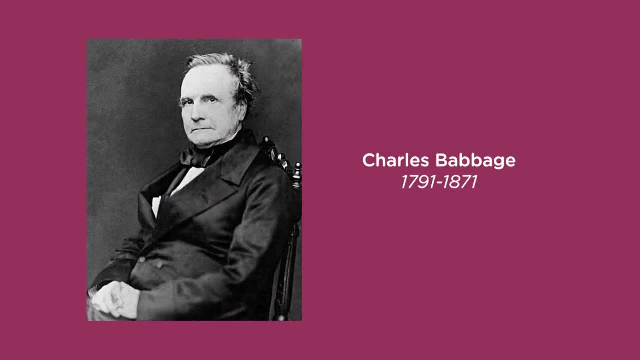 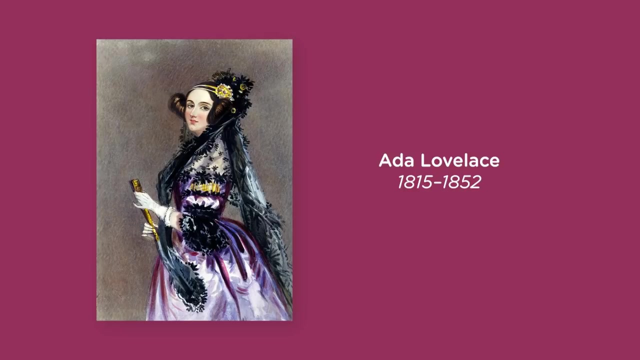 know where you've been. Charles Babbage is widely considered the father of the computer. Babbage is credited with inventing the first mechanical computers in the 1800s. Mathematician Ada Lovelace is credited with publishing the first computer program in the 1840s, designed for use on one of Babbage's early machines. 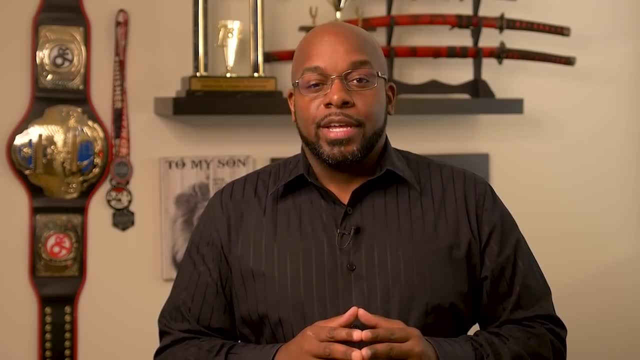 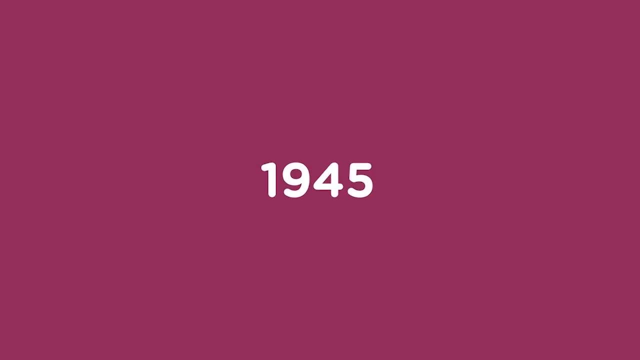 But even after Ada Lovelace wrote the first program, it would still be over a century before the first large-scale programmable computer was introduced. Built in 1945, the ENIAC was commissioned at the University of Pennsylvania in Philadelphia. The ENIAC was nine. 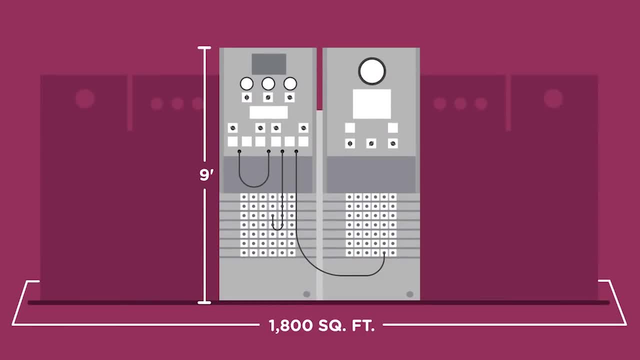 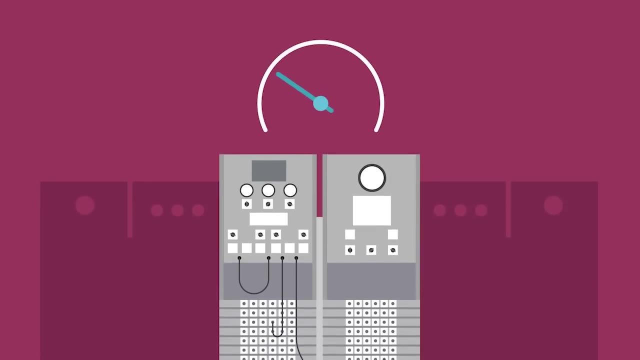 feet tall, covered 1800 square feet, weighed nearly 30 tons and cost $500,000.. Adjusted for inflation, that's over $7 million in 2021.. It's Sported an impressive clock speed of 100,000 cycles per second. 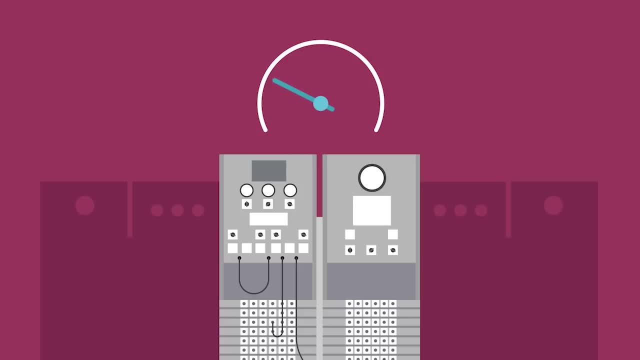 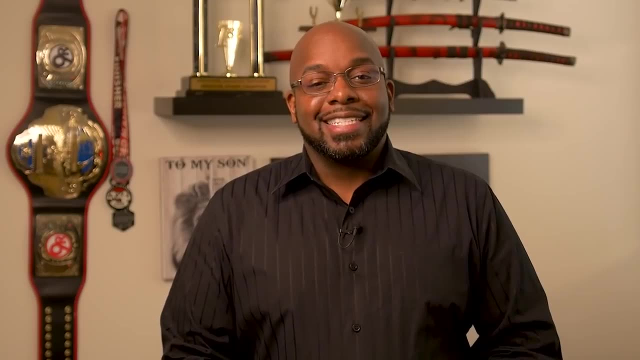 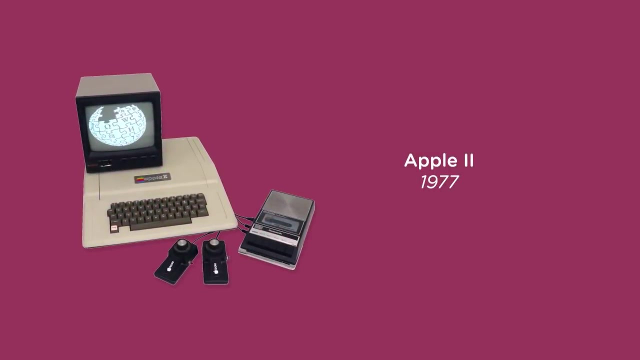 In other words, it could add two large numbers together five thousand times in one second. The first personal computers were introduced in 1977 by three different companies known as the Trinity. One of those computers, the Apple II, helped launch the Apple Computer Company, known today for the MacBook line of laptop computers. 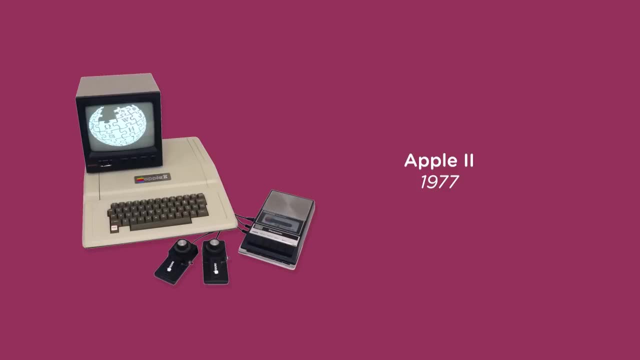 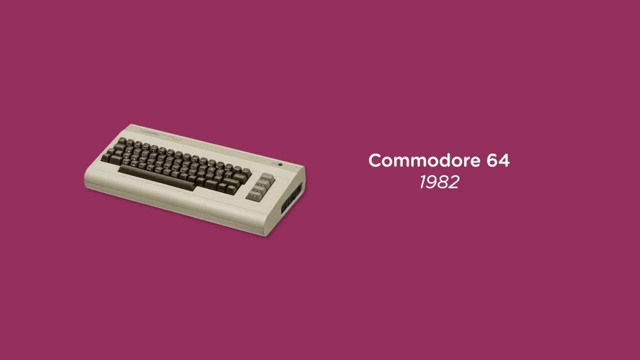 and and mobile devices such as the iPhone and the iPad. In 1982, the Commodore 64 was born, Selling 17 million units. the Commodore 64 still holds the title as the best-selling computer of all time. Fast forward to now. 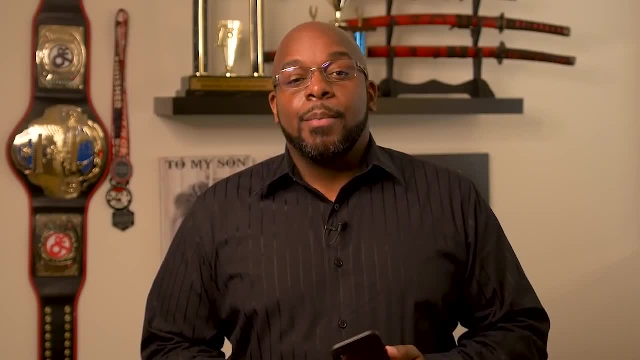 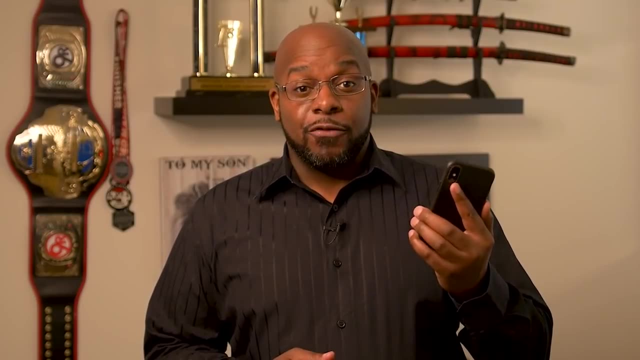 The iPhone X was released in 2017.. Compared to the 30-ton basement-sized ENIAC, the iPhone X weighs less than half a pound and fits comfortably in your hand. It has a clock speed of 2.1 billion cycles per second. 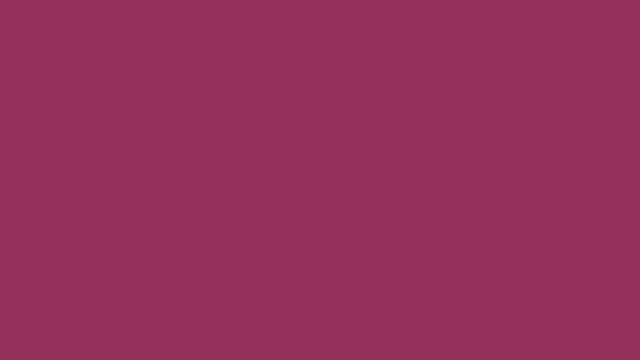 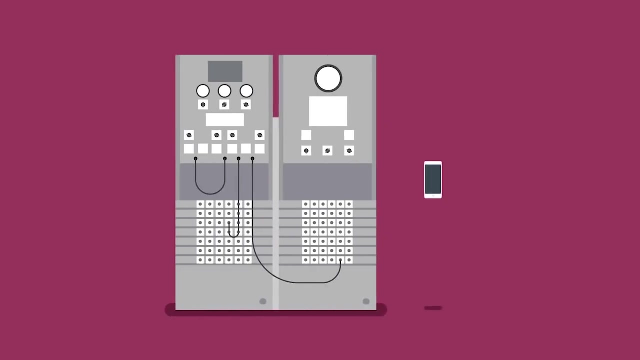 and costs about $1,000 at the time of its launch. To put that in perspective, the iPhone is over 20,000 times faster than the ENIAC and a tiny fraction of its size and cost. In fact, the mobile devices of today can do things. 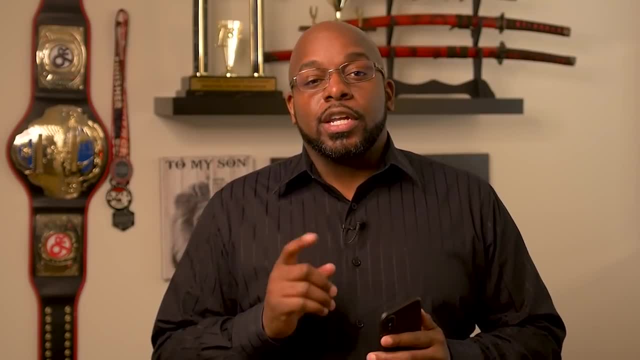 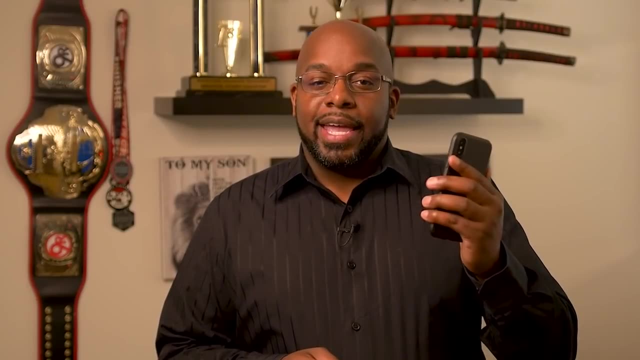 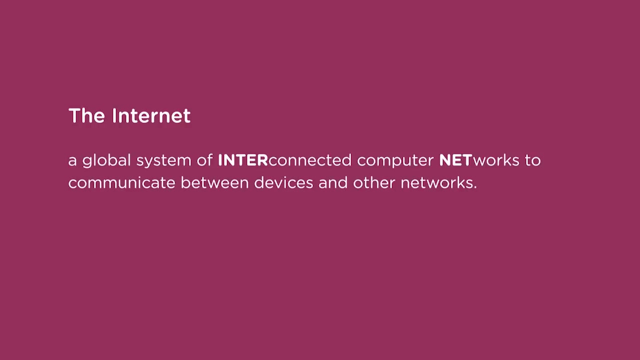 that even the most powerful computers of 20 years ago couldn't accomplish, For instance. I have access to the internet and the worldwide web right in the palm of my hand. Let's talk about them. The internet is a global system of interconnected computer networks. 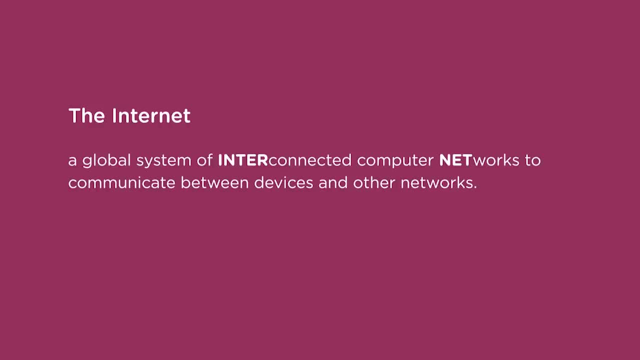 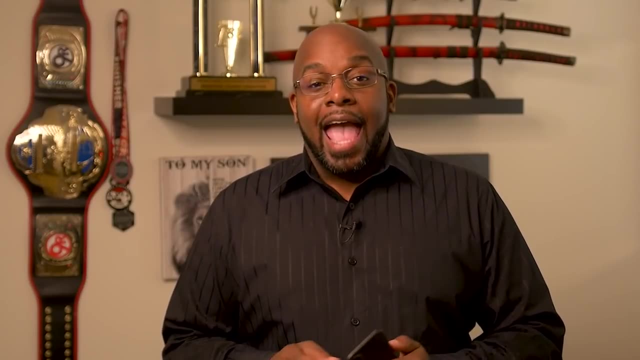 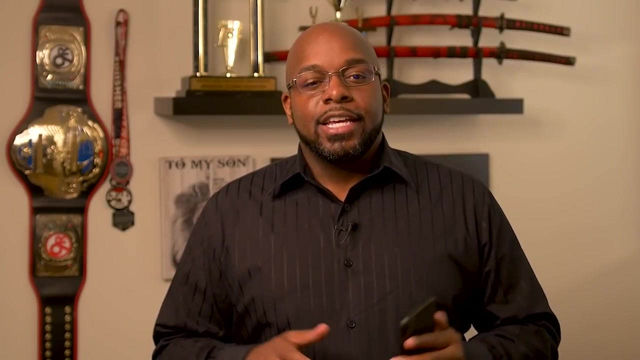 to communicate between devices and other networks. In other words, the internet is a network of networks that consists of public, private, academic, business and government networks. has completely reshaped the way we communicate, shop, learn and conduct business The World Wide. 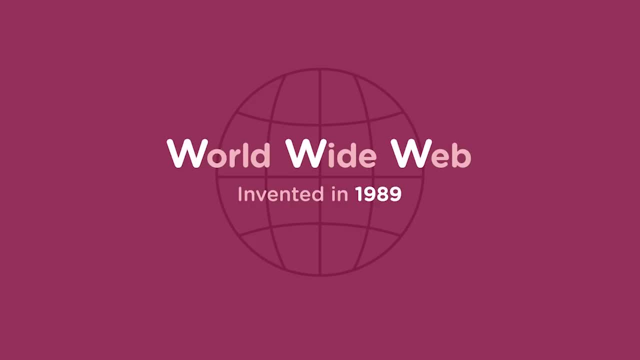 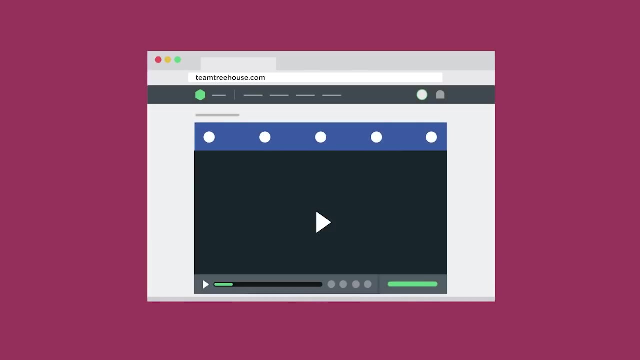 Web was invented by Tim Berners-Lee in 1989, and the public was first granted access to this new network in 1991.. The web allows us to access information on the internet using a web browser. I can visit a website like teamtreehousecom and click on hyperlinks to access other web pages. 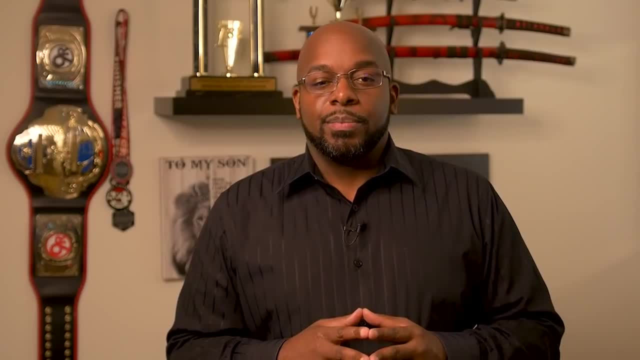 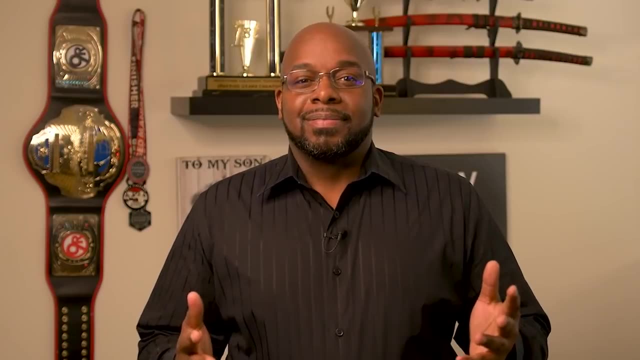 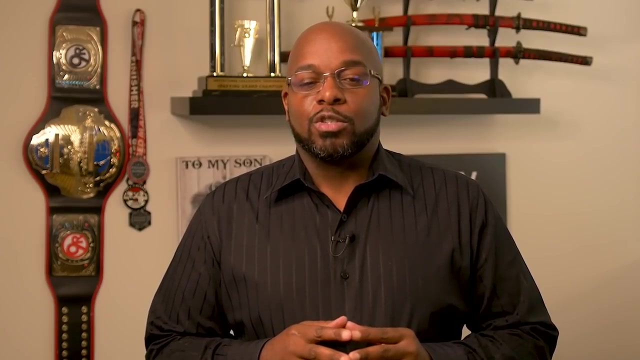 In the next video we talk about different computer components: Hardware, software, storage. oh my, Stay tuned. Welcome. In this video we'll introduce you to different components of the computer. We will define and provide examples of hardware, software, input, output and storage. 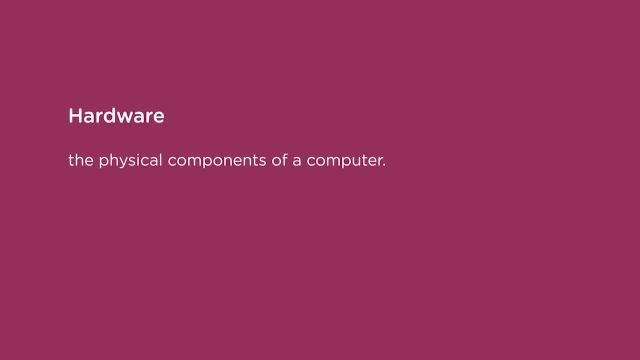 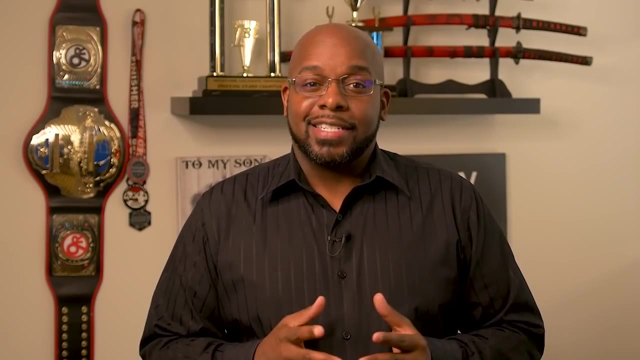 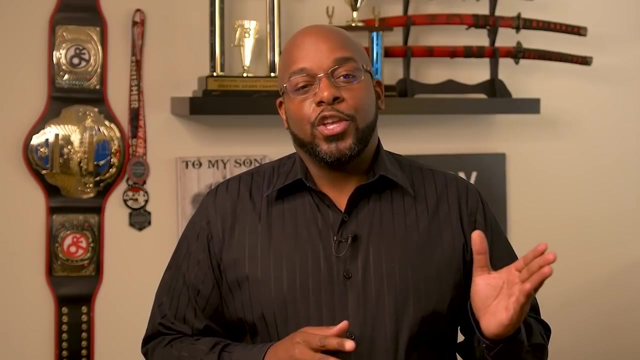 Let's start with hardware. Hardware refers to the physical components of a computer, In other words, the parts you can actually touch, And, yes, they are typically hard. The main brain of a computer consists of the CPU and RAM, or the main memory. 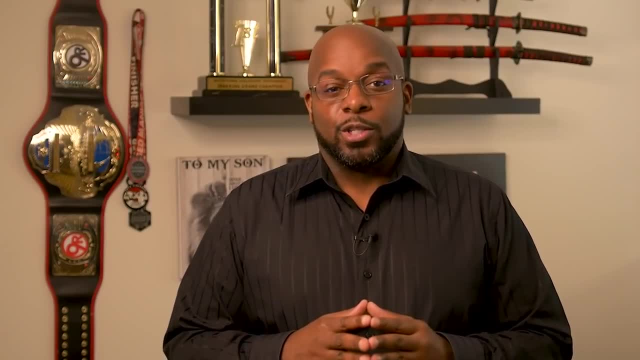 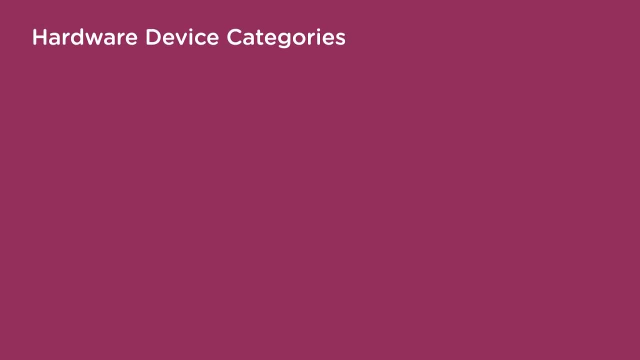 I can teach an entire course on how these components work, but just know that all of the parts of the computer communicate with the main brain. Outside of that, we can divide hardware into three device categories: Input, output and storage. An input device is hardware. 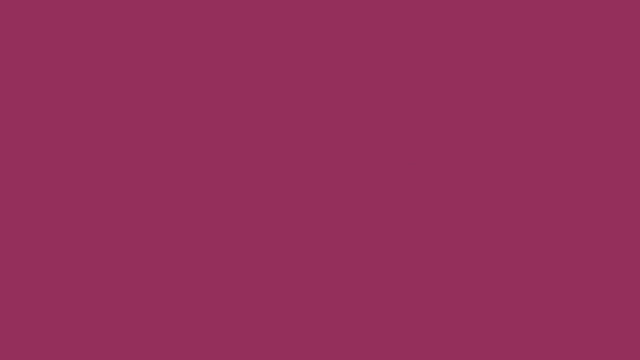 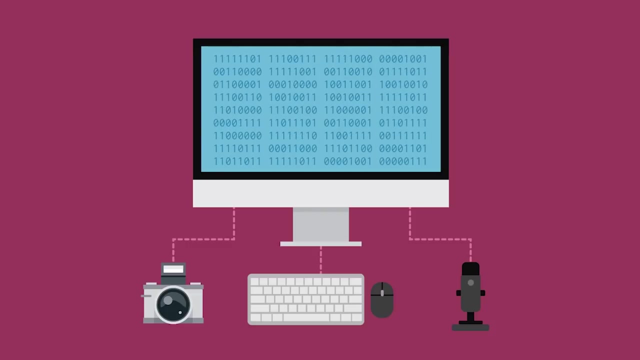 that provides data to a computer. For example, you may use a keyboard and mouse to enter data into a word processing application, a camera to take photographs and a microphone to record audio. The computer receives this information and converts it into data it can use. 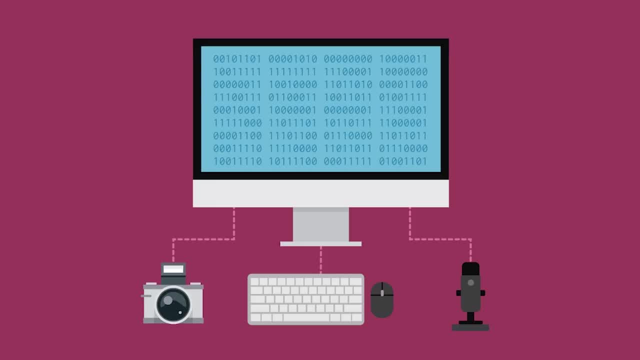 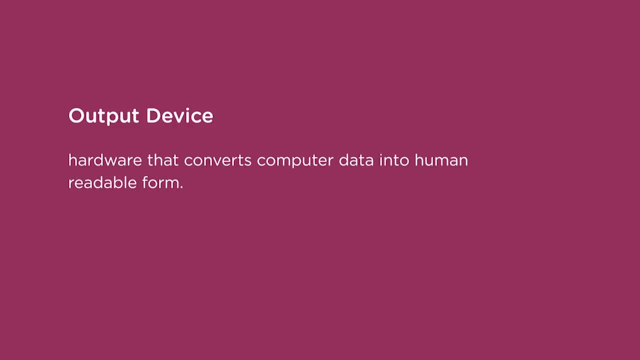 namely a series of zeros and ones called binary, which we'll dig into in the next video. An output device is hardware that converts computer data into human readable form. For example, a screen displays text and images. a printer provides a physical paper output for later use. 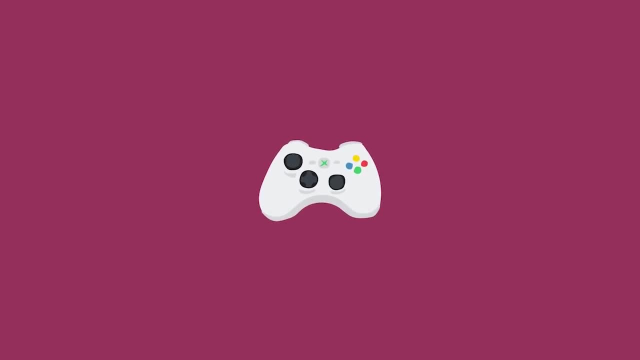 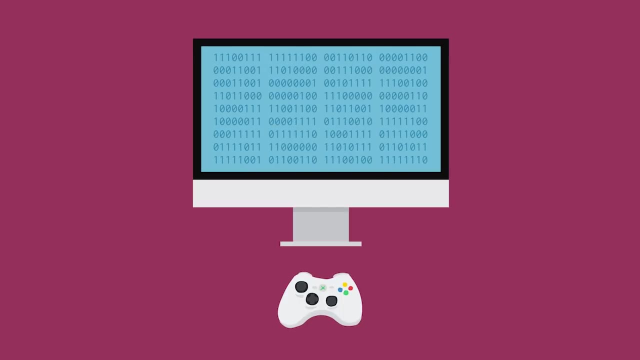 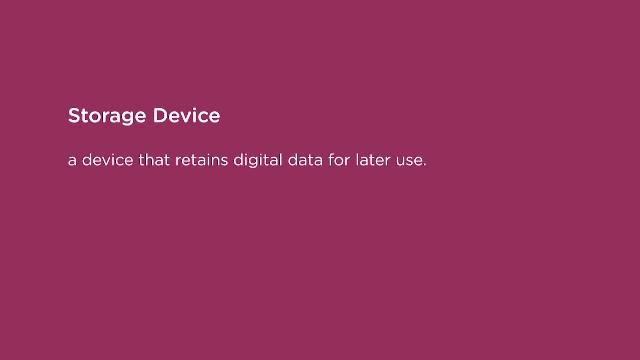 speakers offer audio feedback and your video game controller provides tactile feedback whenever it vibrates in your hand. The computer only sees zeros and ones, but it converts it back to information that humans can understand. A storage device retains digital data for later use. 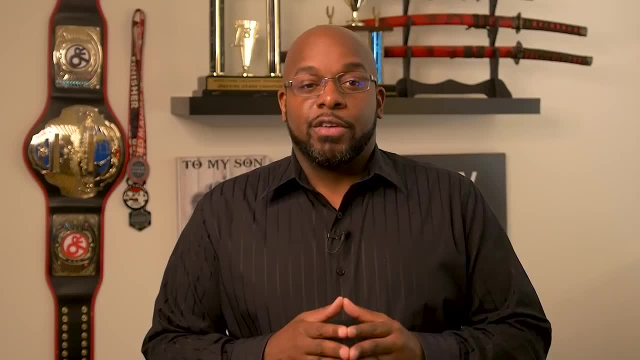 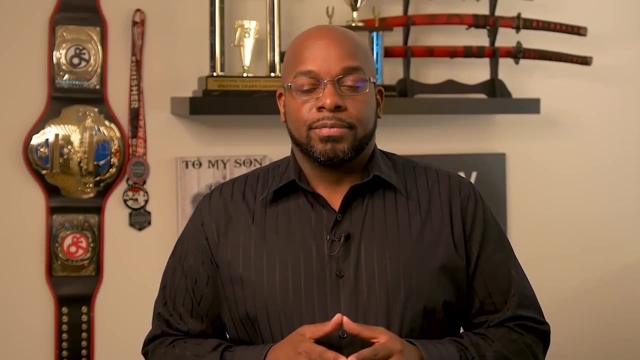 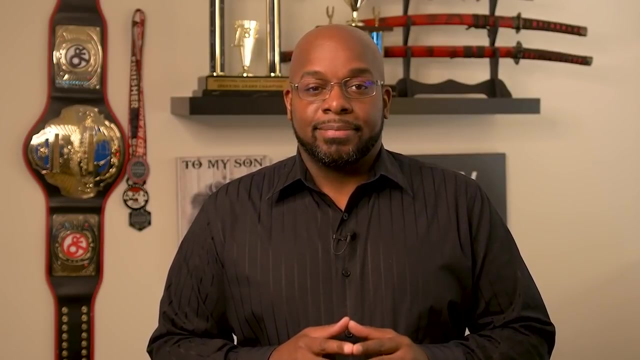 I briefly mentioned RAM, which serves as the primary memory of the computer. However, main memory is volatile, which means it's lost when your computer is powered off. For this reason, we rely on secondary and tertiary storage to save information permanently. Secondary storage can refer to the hard drive. 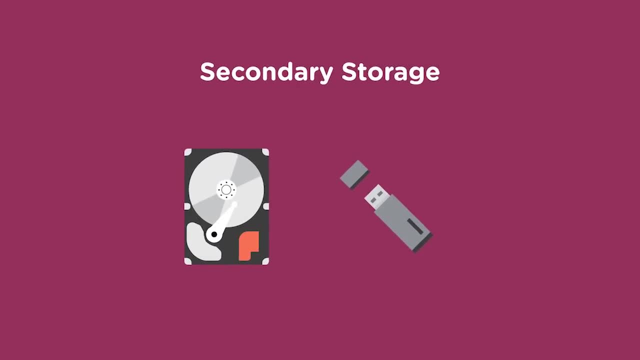 that is often housed inside your device, a flash drive that plugs directly into a USB port of your computer, and even CD and DVD-ROM discs that are historically popular for distributing music, movies and software. Tertiary storage is also known as cloud storage. 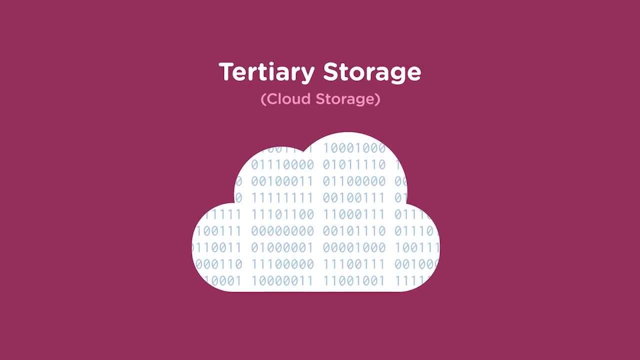 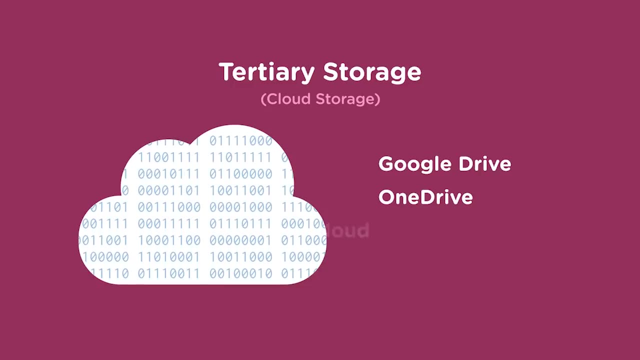 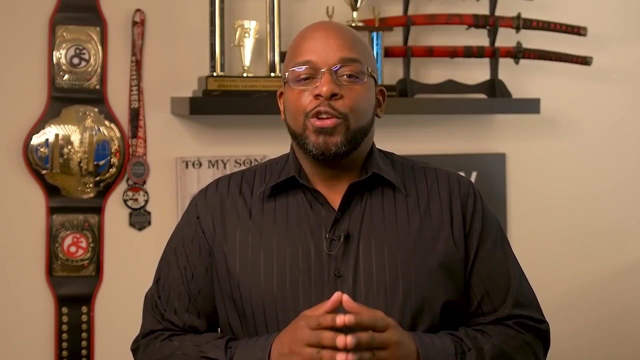 This means that the data is stored somewhere different from your physical location. Examples of cloud storage are, for example, Google Drive, OneDrive by Microsoft, iCloud by Apple and Amazon Web Services or AWS, If you use any of these services. 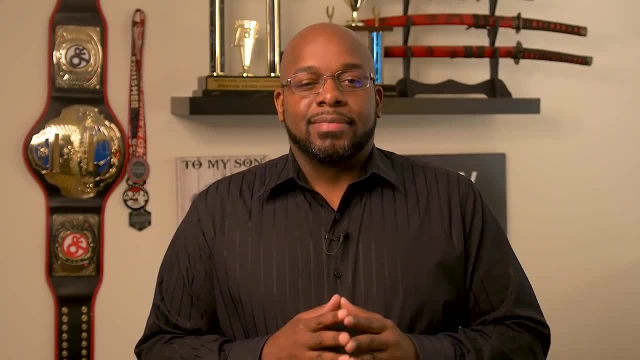 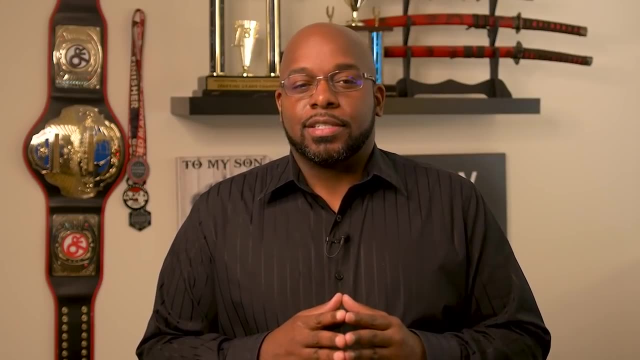 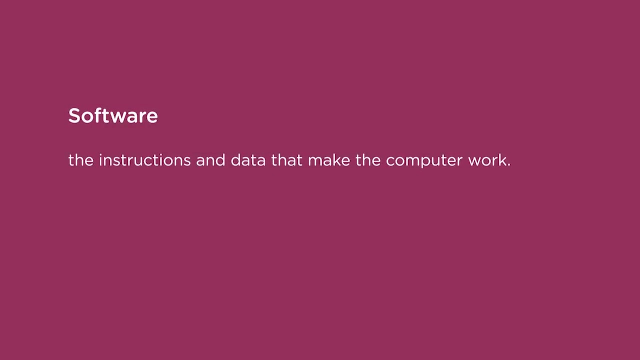 you're saving data in the cloud. I could go into a lot more detail about hardware. However, without software, the hardware is pretty useless, So let's talk about it. Software refers to the instructions and data that make the computer work, such as system software. 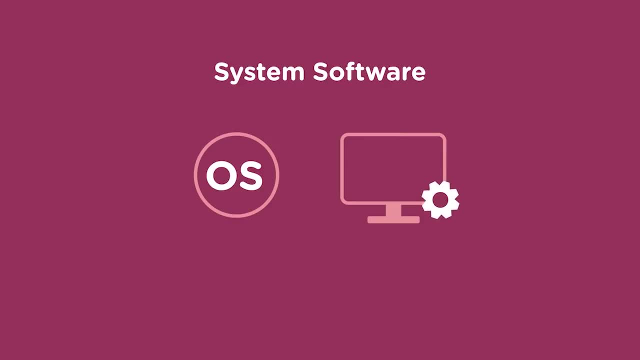 which includes the operating system and device drivers. This is the boring stuff that runs in the background. Think of it like this: If your house is the hardware, the system, software would be the plumbing and electrical system. Sometimes you take it for granted, but if it breaks down, 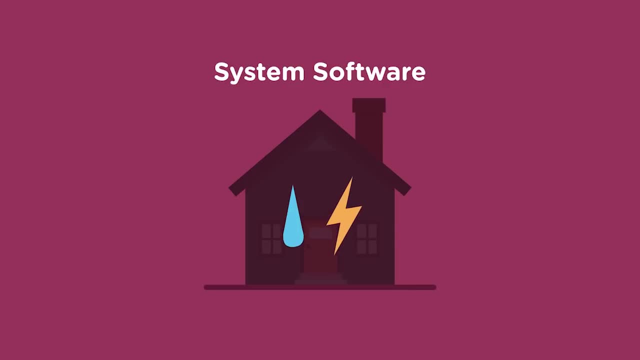 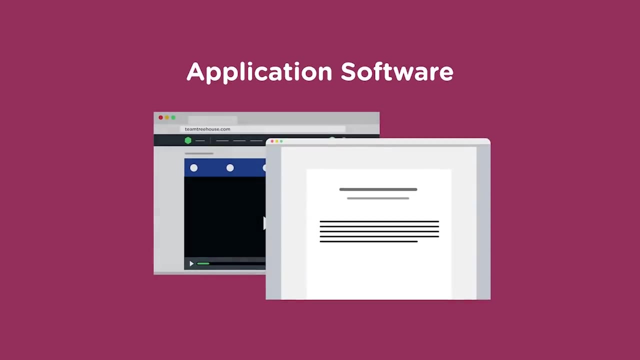 you go out of your way to get it fixed. You may be more familiar with application software. This includes the web browser you use to access treehouse content, the word processor to write letters, the spreadsheet application to manage your budget and the apps on your smartphone. 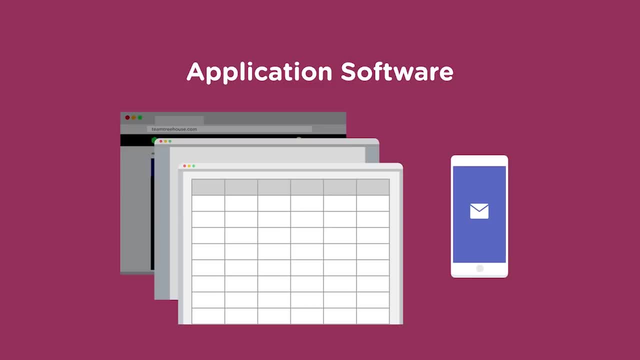 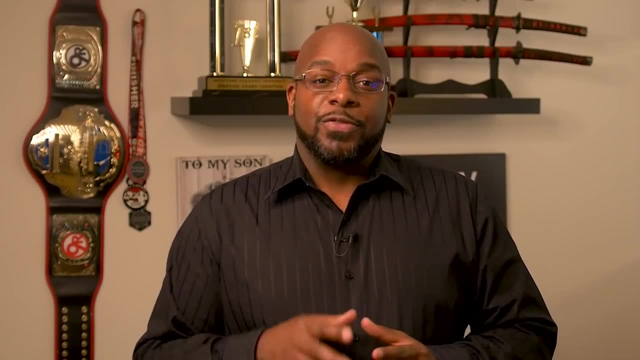 Throughout your journey. here you may learn how to design application software for use on your laptop, favorite web browser and even your mobile phone. In the next video, we'll learn about bits, bytes and the prefixes used for large amounts of data. 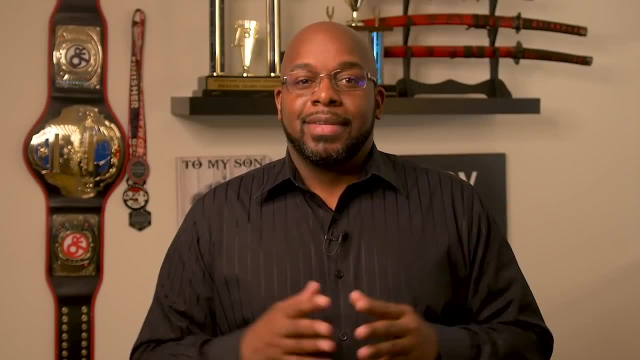 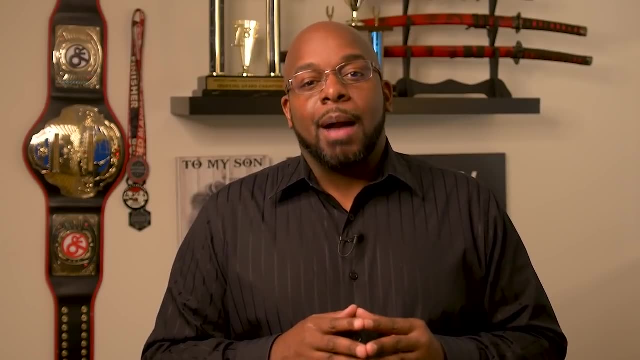 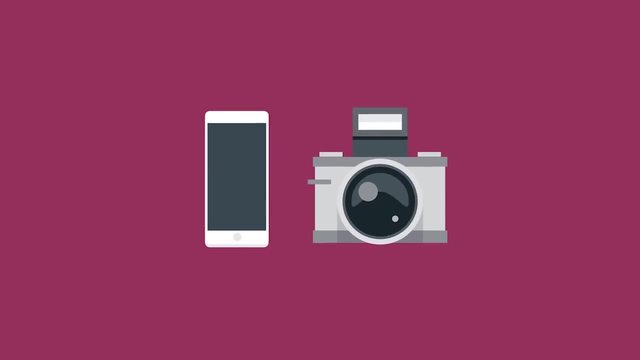 See you soon. Welcome. In this video I will introduce you to the terms bit and byte. We will then identify some common prefixes used for larger values and what they mean to you. You may have a mobile phone or a digital camera that uses very small storage cards. 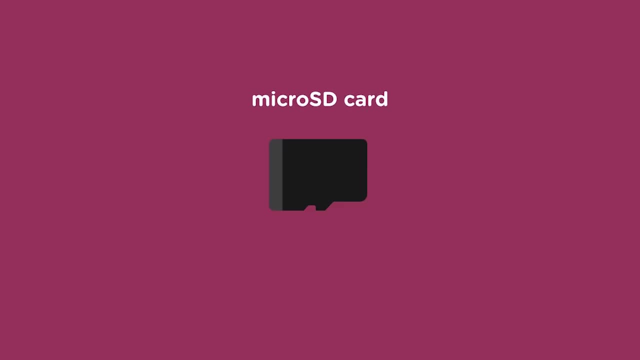 This is called a micro SD card and it's small enough to fit on your thumb 10 years ago. you can purchase one of these cards and you can take hundreds of high-resolution cards. and you can take hundreds of high-resolution photographs. 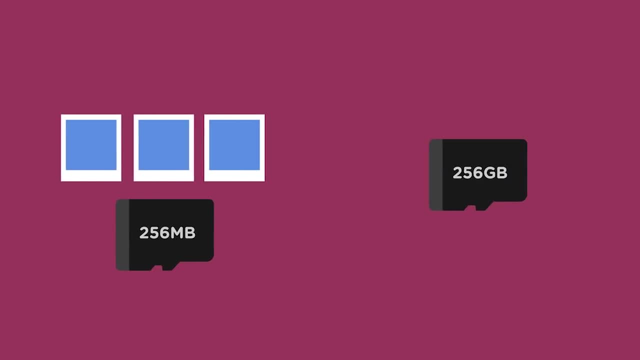 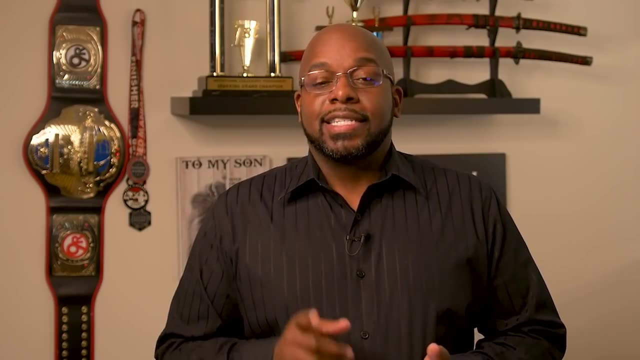 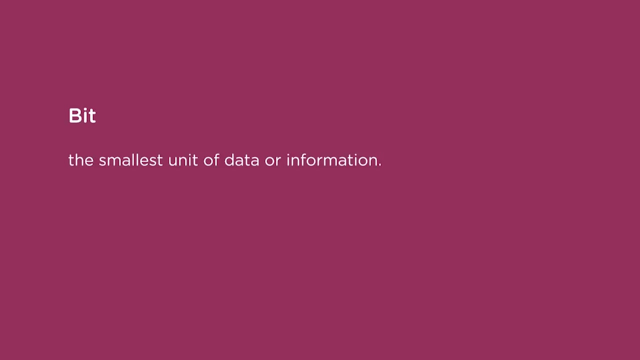 before running out of space. Today, you can buy a thumb-sized card and take hundreds of thousands of photographs. How is this possible? To start, let's get a better understanding of bits and bytes. A bit is the smallest unit of data or information. 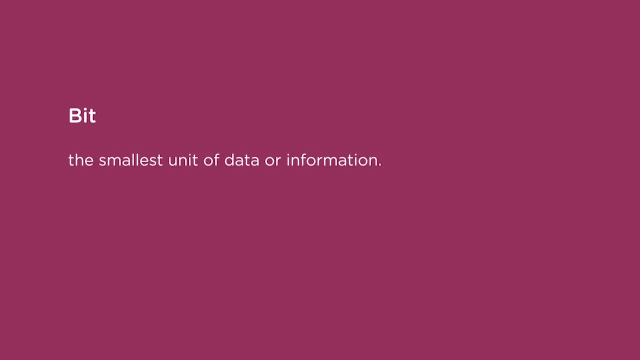 It is short for binary digit, which means it is either one or zero. You can think of this as a light switch in the on or off position, or the answer to a yes-no question, as true or false. A byte commonly consists of eight bits. 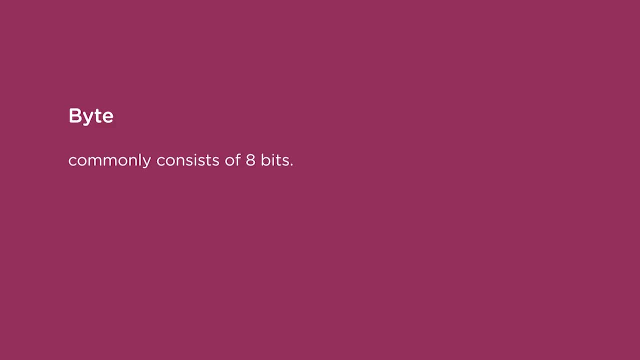 Historically, it was used to store a single character, like the letter R or the number 7.. We usually refer to a file size in terms of bytes. For example, this Python icon is 259 bytes. My resume stored as a word processing file. 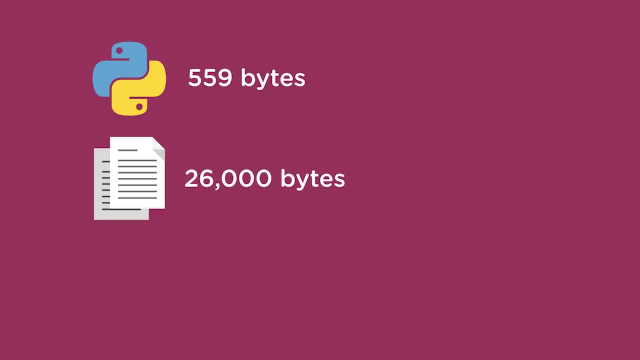 is 26,000 bytes. The movie Hidden Figures stored on a Blu-ray disc is more than 39 billion bytes. There is a better way to refer to these large numbers by using different prefixes before the word byte. For example, kilo means 1,000,. 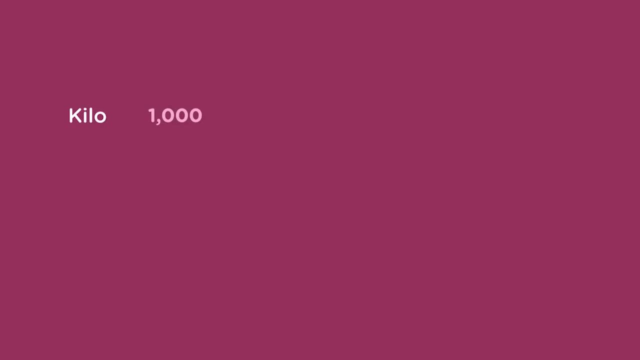 or one, followed by three zeros. You may have heard of kilo before. A kilogram means 1,000 grams, A kilometer or kilometer means 1,000 meters. So instead of 26,000 bytes, I would say that my resume is 26 kilobytes. 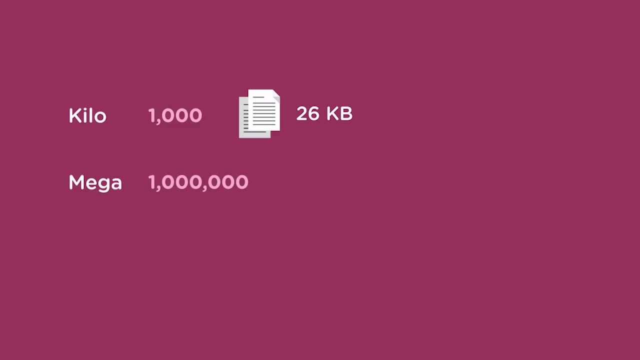 Mega means one million, or one followed by six zeros. My favorite song stored on a portable music player is 4.7 megabytes. Giga means one billion, or one followed by nine zeros. The DVD of Hidden Figures is 39.26 gigabytes. 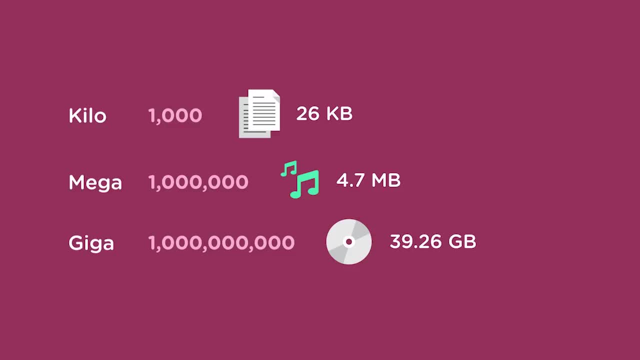 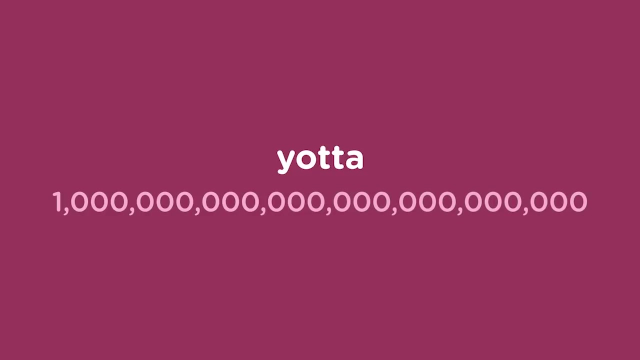 There are more prefixes for even larger values. The largest widely recognized prefix is yata A yata byte is one septillion bytes, or one followed by 24 zeros. This is about 45 trillion bytes. This is about the size of a Blu-ray movie disc. 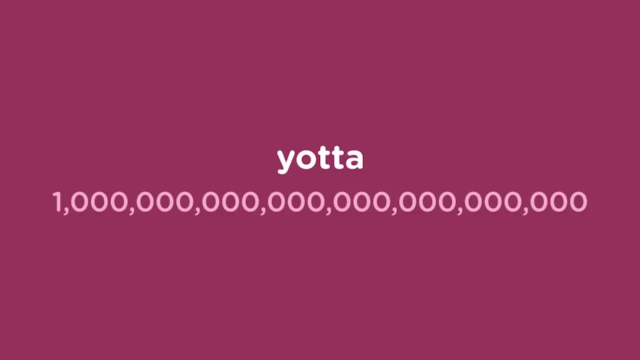 or 1,000 years of worldwide internet traffic. To house one yata byte of data you would need a data center roughly the size of the state of Connecticut. Back to that micro SD card for your phone. Today you can buy a 256 gigabyte card. 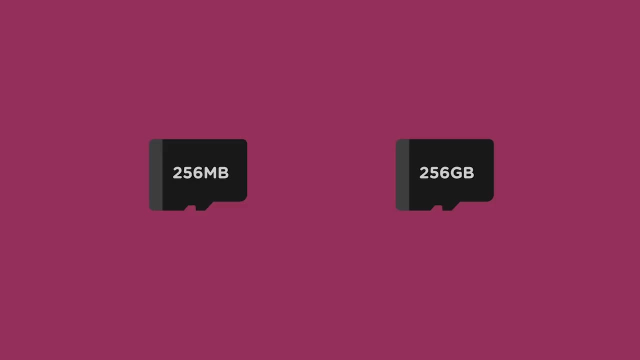 for the same price you would have paid for a 256 megabyte card 10 years ago. The difference is the card you buy today stores 1,000 times the amount of data. In the next video we will discuss the different types of data. 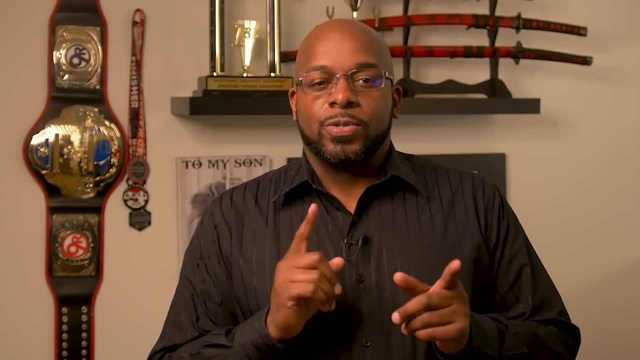 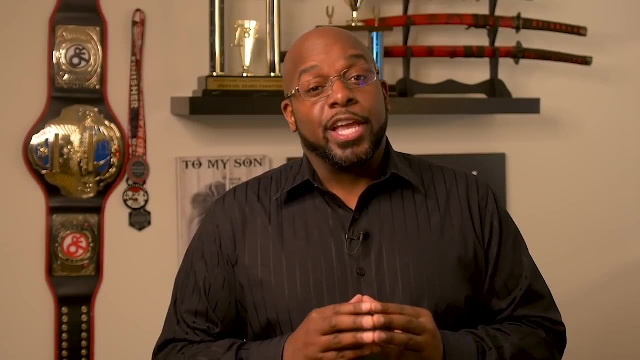 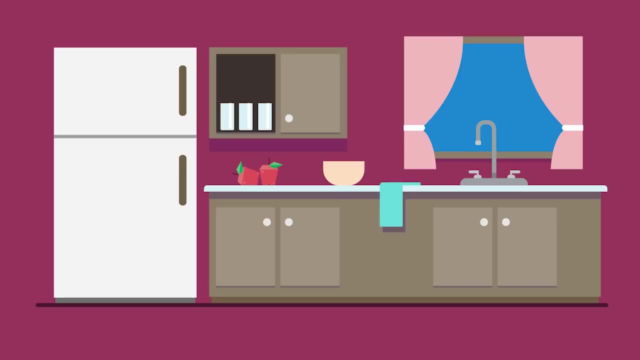 you will use when writing computer programs. Stay tuned, Welcome. In this video we will introduce you to several data types you may encounter in your programming journey. Consider the cabinets in your kitchen When I was growing up: the cabinet next to our refrigerator. 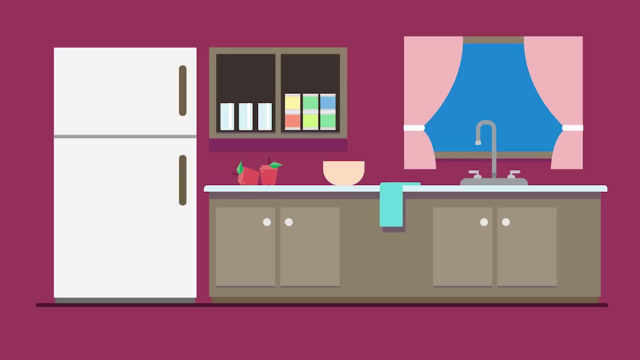 was only for drinking glasses. The one above the countertop was for canned foods. The cabinet under the sink was for cleaning supplies. Now, you would never think to store a drinking glass under the sink, And I learned very quickly not to put the green beans. 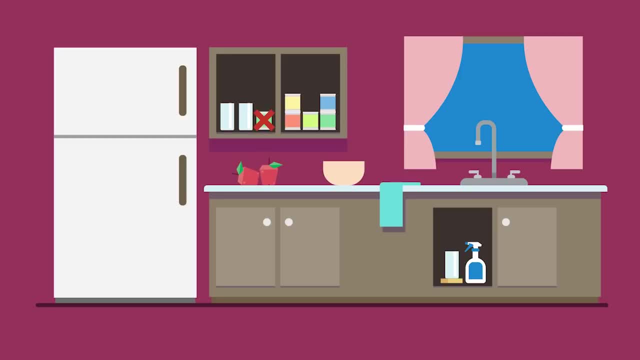 in the cabinet next to the fridge. Think of these kitchen cabinets as data types. Each data type is designated to store one specific type of data. If you break the rule, well, you may get in trouble. Some programming languages allow you to store data. 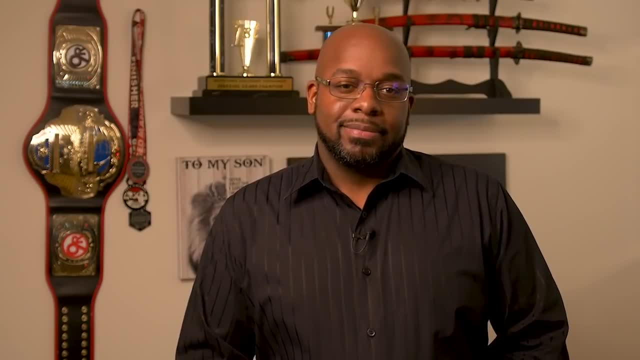 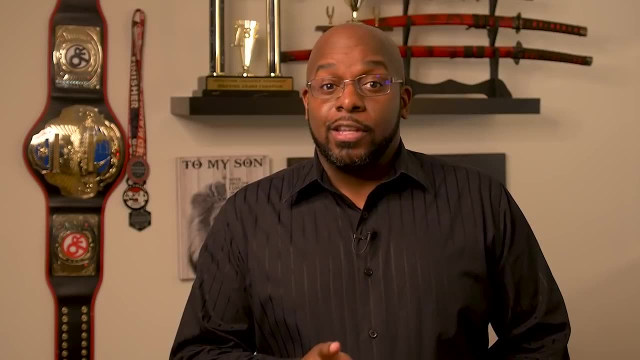 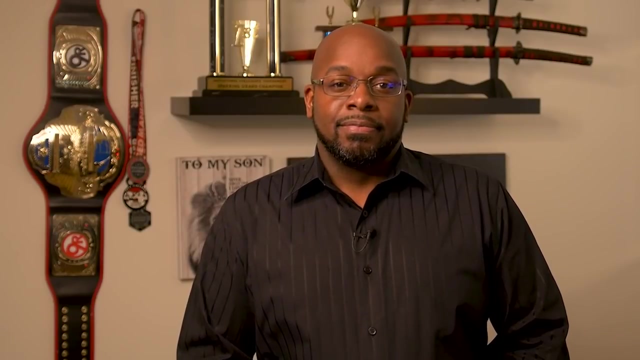 without first identifying its type, like Python. Some languages allow the data's type to change throughout the code, such as JavaScript. Other languages force the programmer to identify the data's type before using it. Talking about you, Java, There are so many different data types. 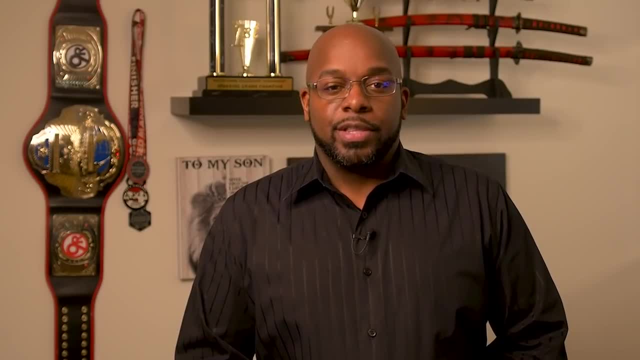 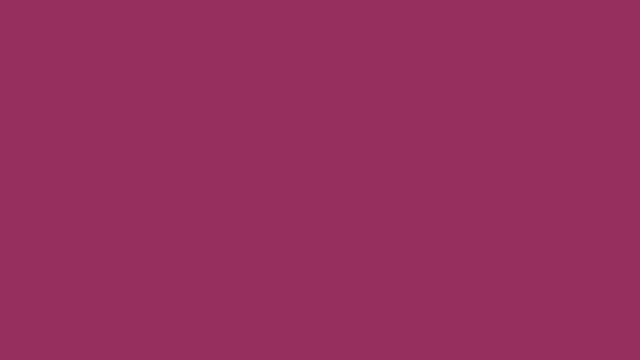 and each programming language has its own rules on how to use them. Regardless of the language, you are likely to encounter one of these three data types. The first is text. It's a combination of letters, numbers and symbols. For example, you can store: 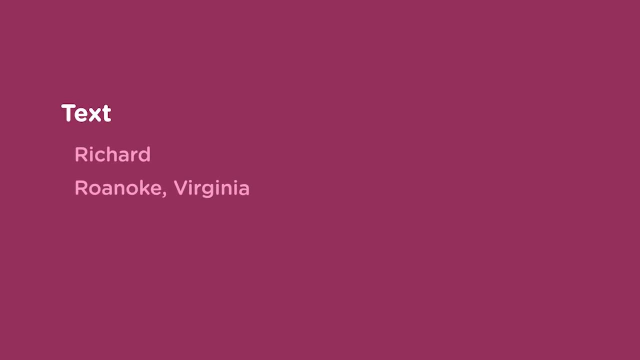 my name Richard, my hometown, Roanoke, Virginia, or a complete sentence: I can be reached at 540-555-1234.. Next is numeric data. The advantage of numeric data is that I can perform mathematical operations. I can store whole numbers. 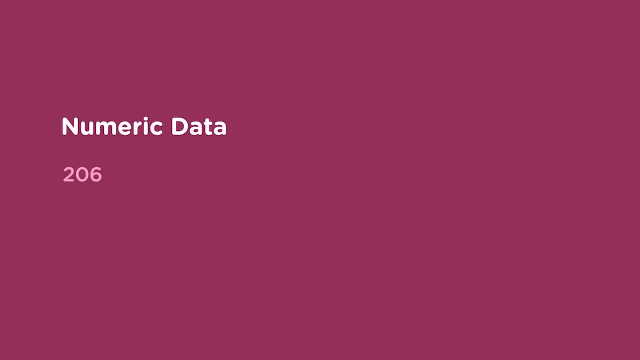 The number of bones in the human body: 206.. Population of a city: 102,345.. Numbers with a decimal point, Pi, rounded to four decimal places: 3.1416.. Ounces of water in a liter: 33.8.. 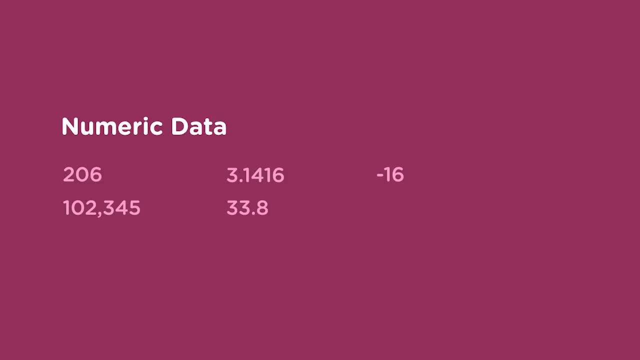 And even negative numbers. Strokes under par in a golf tournament: negative 16.. Absolute zero in Celsius: negative 273.15.. Finally, I can store Boolean values. A Boolean represents the truth value stored as a bit. Remember that a bit. 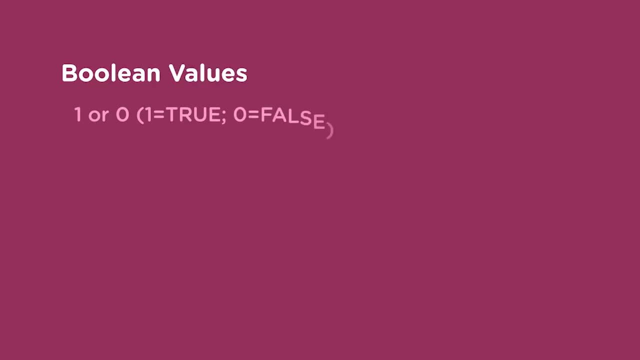 can only be one of two values: true or false, one or zero. One means true, zero means false. Think of a light switch as on or off, or the answer to a question as yes or no. Is the Nile River the longest river in the world? 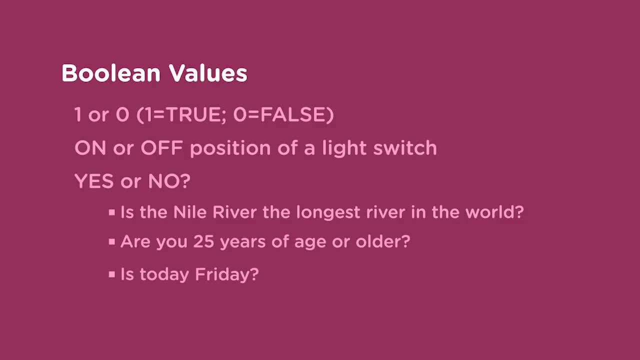 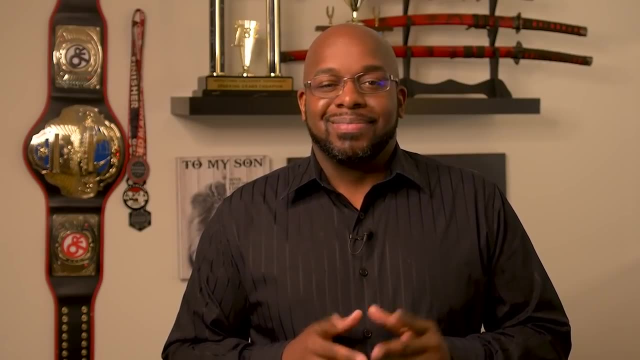 Are you over 25 years of age Is today, Friday. As you write code, you determine how to store and use data in your program. Don't worry, that's a discussion for another time. In the next video I give you a brief introduction to programming. 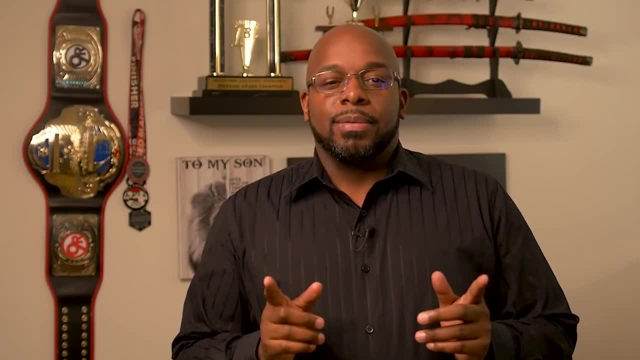 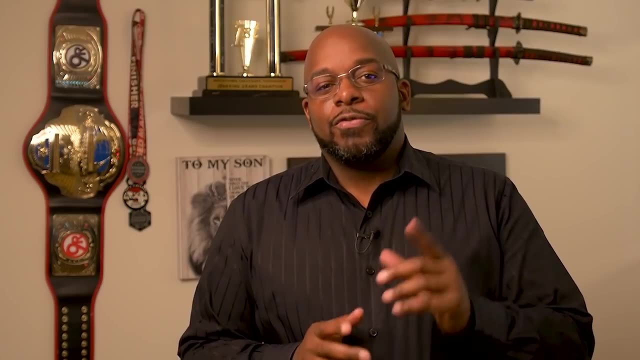 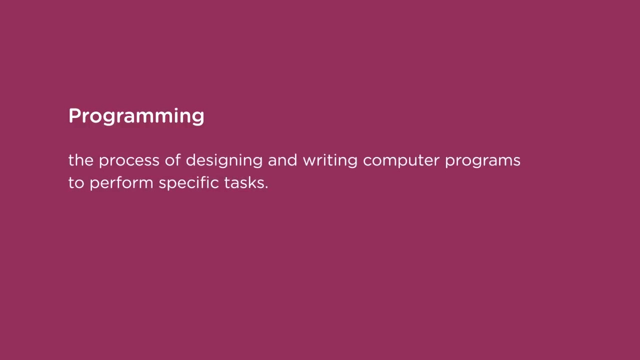 Stay tuned, Welcome. In this video we wrap up your computer science primer with an introduction to computer programming. Let me give you a few definitions. First, what is programming? Programming is the process of designing and writing computer programs to perform specific tasks. 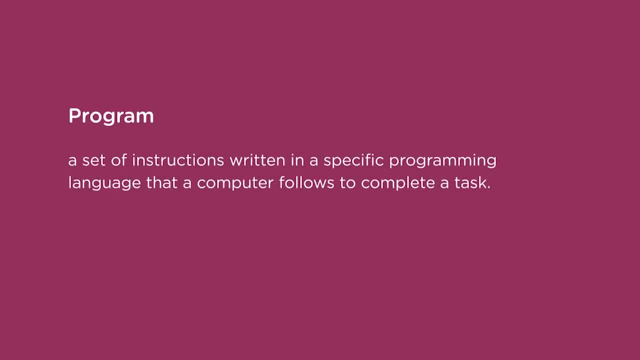 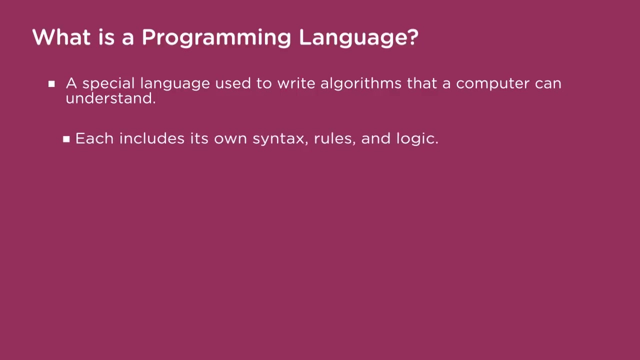 What is a program? A program is a set of instructions, written in a specific programming language, that a computer follows to complete a task. What is a programming language? A programming language is a special language used to write algorithms that a computer can understand. Each programming language has its own syntax. 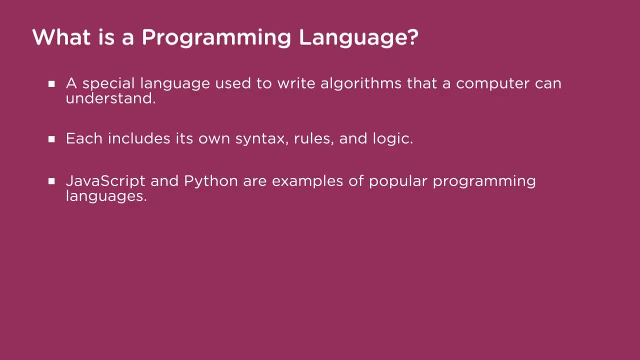 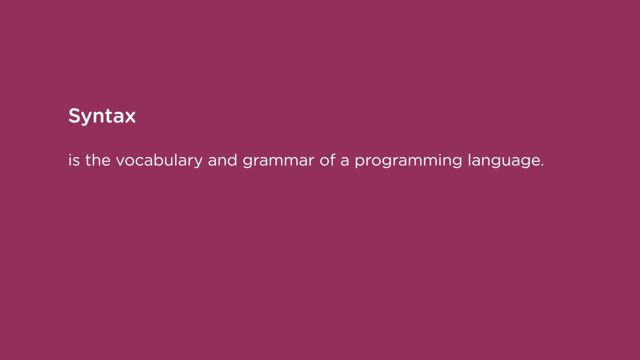 rules and logic. You can learn many different programming languages at Treehouse, like JavaScript and Python. I will explain syntax and algorithm in more detail. Syntax is the vocabulary and grammar of a programming language. It is the special words, commands and punctuation of a language. 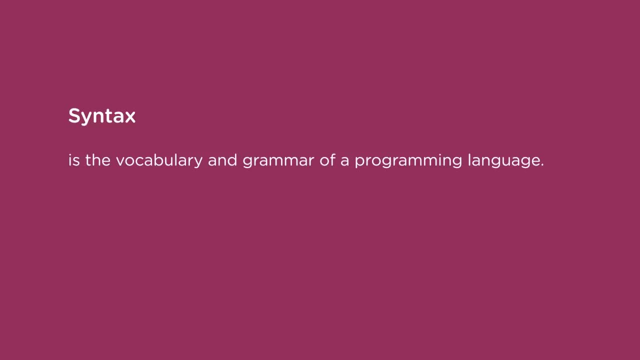 as well as the rules for putting them together to create a program. Let me give you some example sentences in English. Seneca eats lunch at noon. Instagram is my favorite iPhone app. Can Casper cleave the coriander conspicuously? Each statement follows the rules. 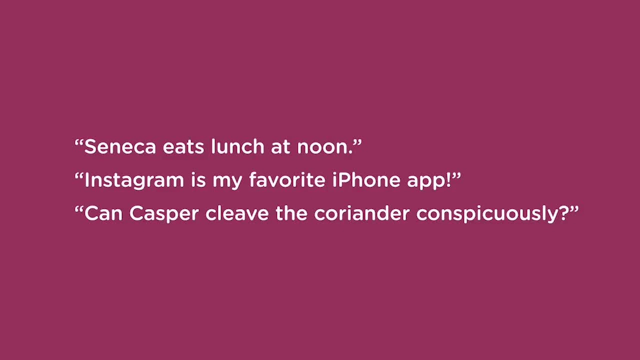 of the English language to form a proper sentence. Even if you don't know all the words in that last example, you probably recognize that I am asking a question about a person's ability to do something. You might think I made up some of the words.